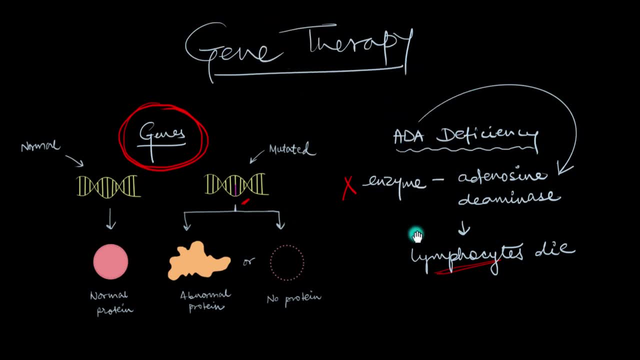 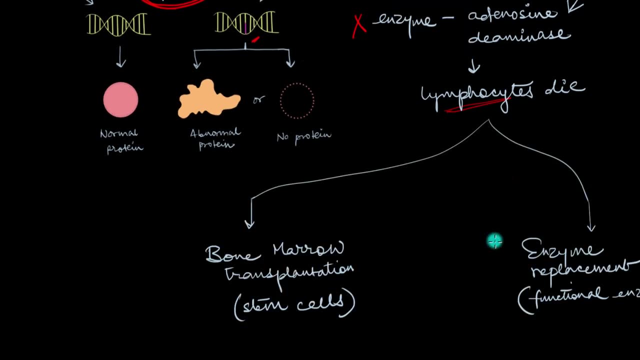 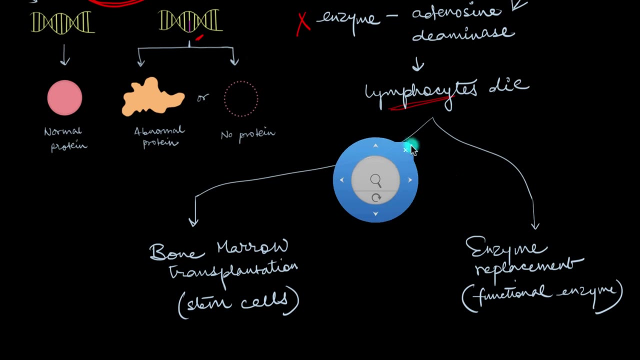 So do we have any solutions for this? Yes, Yes, we do. We do have some solutions for this condition. One of them is bone marrow transplantation. Now, let's move this a little bit to the side. You guys can see it Now. one of the options is called bone marrow transplantation. Now, in this, 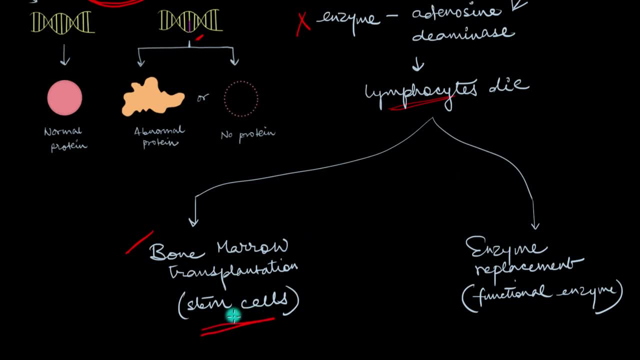 what happens is that you take stem cells from the bone marrow of a healthy person and then you inject it into the patient. Now, stem cells are these cells which grow into a specific type of cell, And the stem cells that we are collecting from the healthy person, these stem cells that 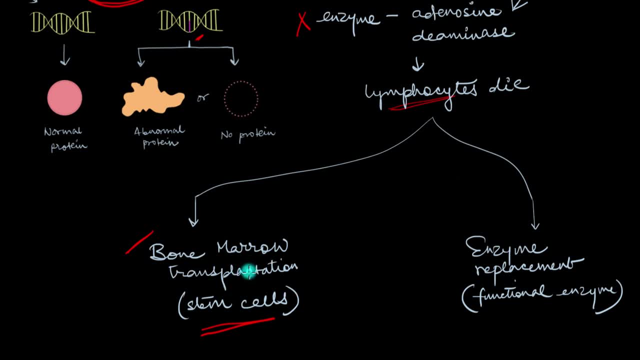 we got from the healthy person. they will grow into new lymphocytes. So we are taking those stem cells and we're injecting it to the patient so that new lymphocytes can be formed in their body. Now, if you don't want to go for 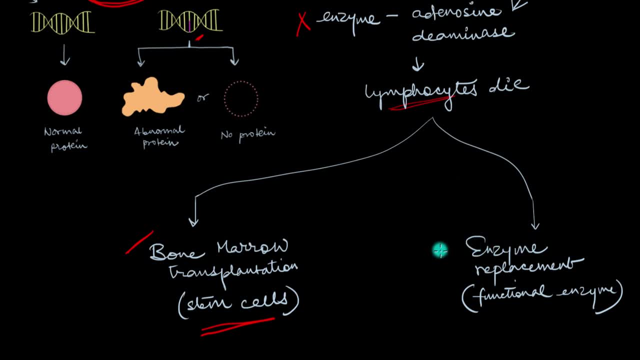 bone marrow transplantation. there's one more option, It's called enzyme replacement theory, in which you inject the functional ADA enzyme directly into the patient. But neither of these. but the problem with these solutions, what is I'll tell you, is that neither of these solutions are well. they're. 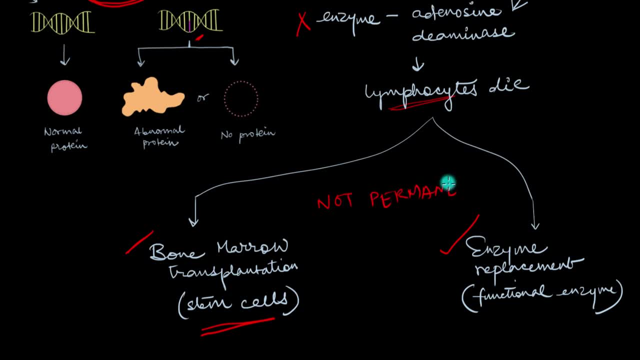 not permanent. So the problem with now? they say that, like some, in some cases bone marrow transplantation has been somewhat permanent, but there is no guarantee for it, given that there's a huge list of side effects And sometimes you don't find the right donor. who's going to donate? 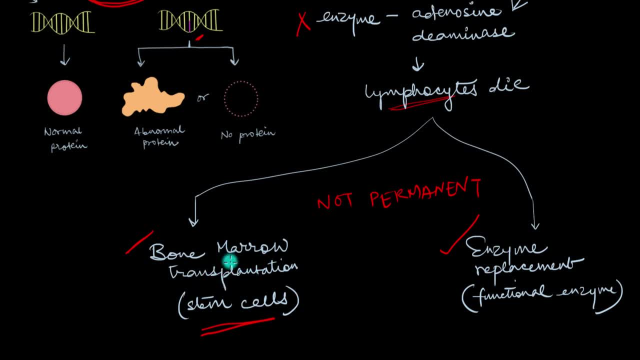 that bone marrow for the transplantation. So, because of a huge number of problems, there's no guarantee that bone marrow transplantation is permanent. And as for enzyme replacement therapy, you have to regularly get that enzyme replaced technically, so you have to get that constantly done. So, because of these non-permanent solutions, 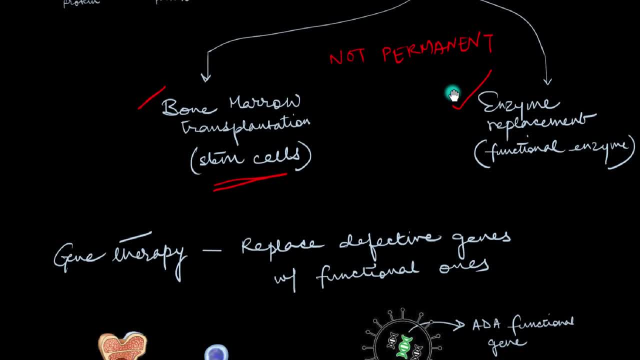 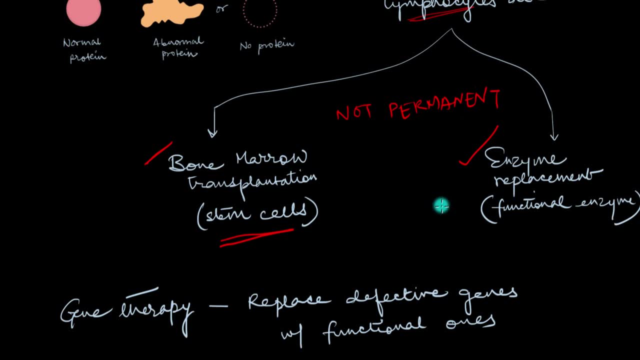 this is where gene therapy kind of comes into the picture. Now, what is gene therapy? That's the first question that probably comes to your mind. Now, gene therapy is this process or a procedure in which you replace the defective genes of something and you replace that with the functional gene. 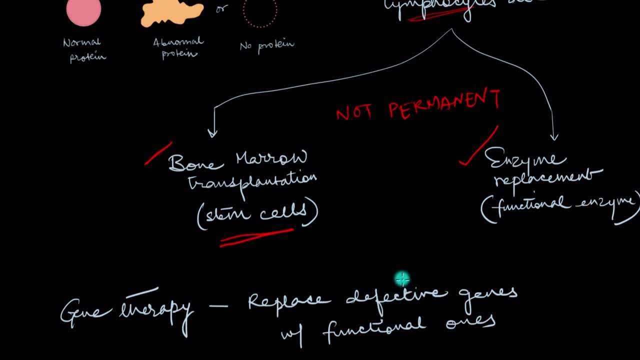 So you replace the defective genes with the functional ones. In this process, what you are essentially going to do is that you will take the functional gene and you will deliver it to the patient, and this new functional gene will compensate for that defective gene and end up producing that gene product which we desperately need. 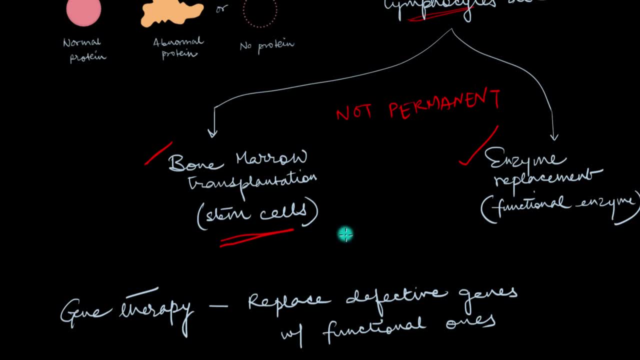 So that is the whole idea behind it. So you can kind of call it that. it's a kind of a correction therapy, where you are correcting that defective gene. So it's a form of correction therapy in one way. But now the main question arises is probably that: 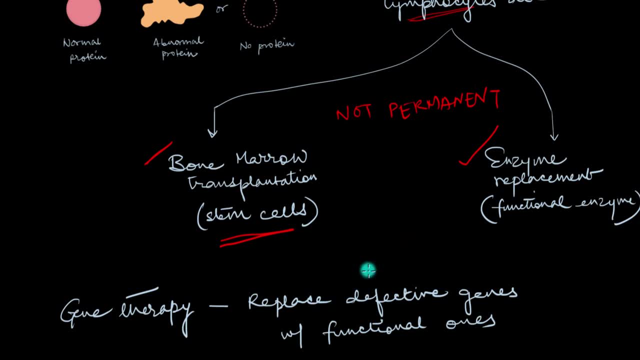 how are you going to do something like that? How are you going to pick out a gene and then insert it into that another person and then also make sure that that gene works perfectly in that person, right? So how exactly do you carry out something so complicated? 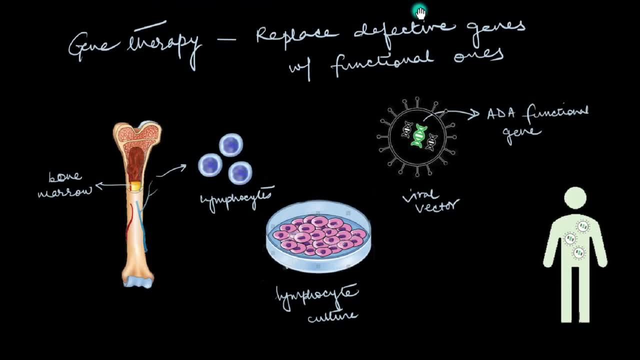 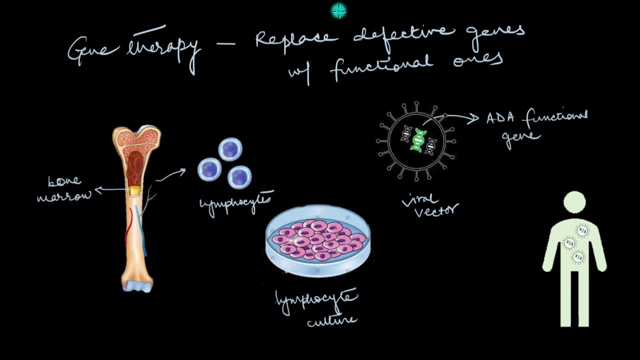 Now, ADA deficiency is one of the very first diseases where this gene therapy method was used for the first time. It's already figured out by now, but I'm mentioning it once again so that we're pretty clear about it: ADA deficiency: this disease is caused due to a mutation, like I said in the beginning. 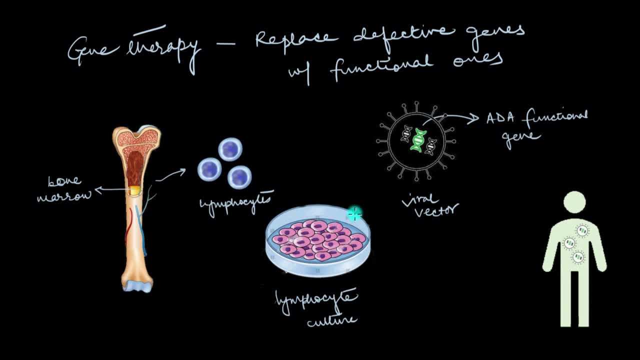 like any tiny change can lead to huge, devastating consequences. So ADA deficiency is also a result of a mutated gene, and gene therapy seemed to be the perfect. and this disease seemed to be the perfect place where gene therapy could be used for the first time, and the first one would be the gene therapy. 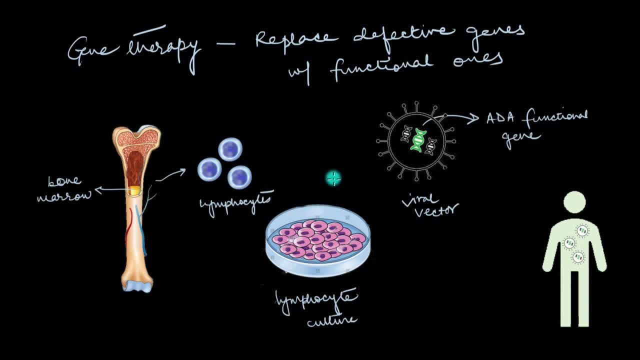 So the approach that they used for ADA gene therapy is something called an ex vivo approach, which literally is like, if you translate this in to out of the living, so what they essentially do, or what they really do in this process, in this ex vivo approach, is that they take: 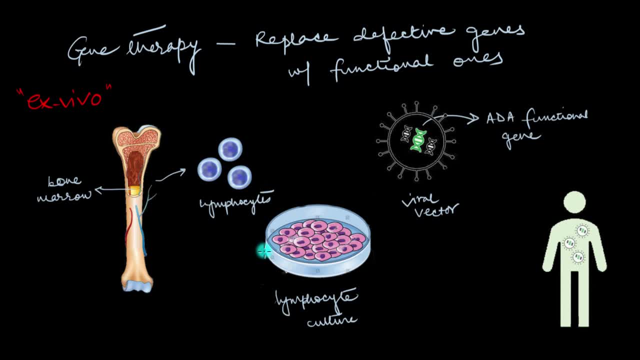 extract it from the patient and then they modify them outside in a culture, like in a plate or in a culture of some sort, and they modify it and then they kind of inject it back into the person. so it's out of the living, outside the living body. that's why it's called the ex vivo approach. so 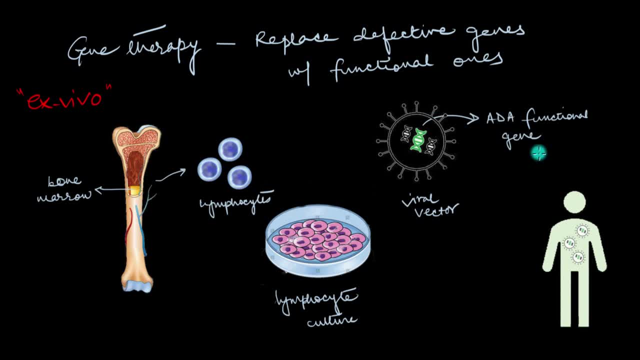 here. what they are going to do is that they will extract the lymphocytes from the bone marrow of the patient, and they're going to then culture it separately in artificial conditions and allow these lymphocyte cells to multiply and grow, and then what they are going to do is: now they're 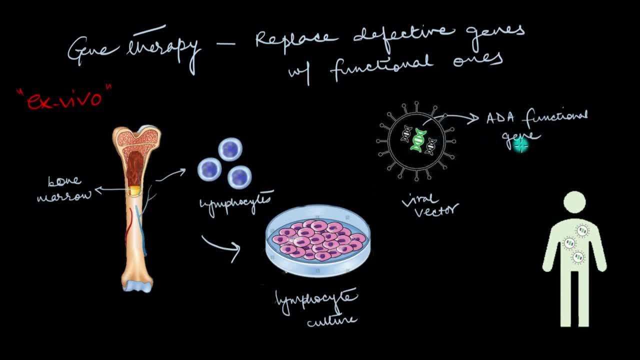 going to add a functional copy of this ada gene. so you can see this green colored gene right over here. let's change the color again. so this, this one, this is the functional ada gene, the functional copy that we have, and we are going to insert this functional gene into the cultured cells that we have the cultured lymphocytes with. 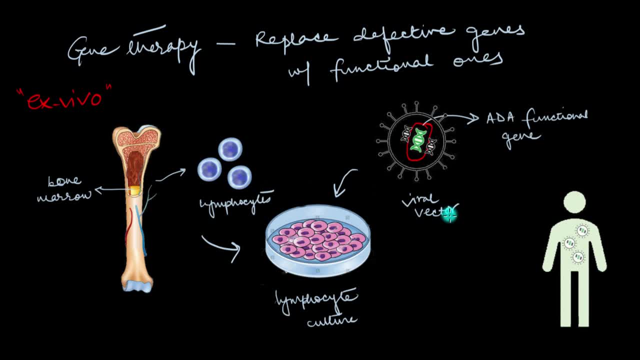 the help of a viral vector. wait, what now? why? you heard me viruses. we use viruses as, or viral vectors like as vehicles to transfer the gene. but the question is: are they safe? is it safe to use a virus as a gene? well, they can be. whenever you use a virus as a vector of some sort, you kind of get rid of. 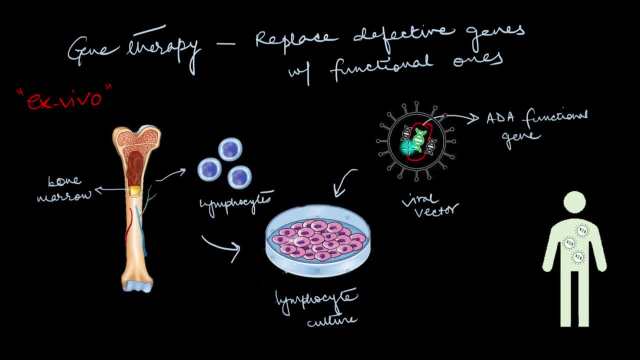 all the harmful genes that can possibly cause some kind of complication in us, that can possibly harm us. so you get rid of all of those viral genes. but the problem is that despite doing something like that, in some cases these viral vectors have known to cause leukemia for some reason in some cases in some patients. so we couldn't have that if we wanted to use viruses. 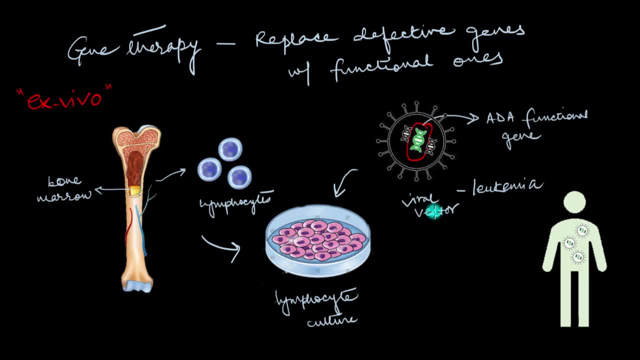 as vectors, we cannot have any kind of underlying complication that can arise from this virus or this viral vector. so what scientists did? they altered these viral vectors in such a way that they don't cause any form of cancer or leukemia, or anything else for that matter. so once they had altered these, 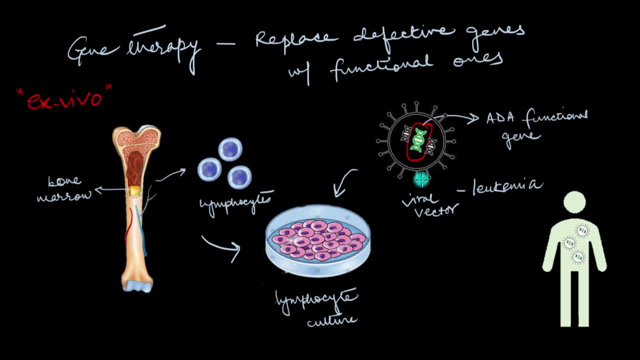 viral vectors. so they kind of got rid of that extra problem that they kept facing. Once these viral vectors have inserted the functional ADA gene into the cultured lymphocytes, we now take these, now modified. so these cells are now modified. wait, let's use a different. 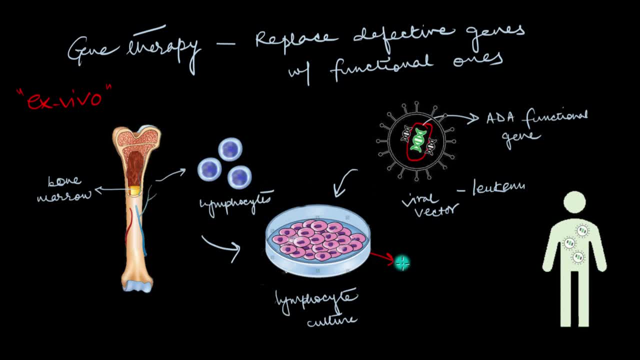 colour, so we'll know. So these cells, right here, they are now modified. So we now take these modified lymphocyte cells and we inject them into the patient. Now, what will happen when these lymphocytes are injected into the person is now that every 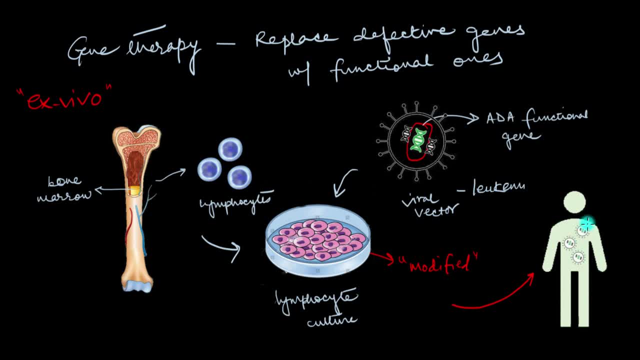 single time a new cell is formed, there will be this new functional gene copy that we had added earlier. So every time the cell replicates, or it grows or it multiplies, then all of those cells will have this new function And because of that the ADA enzyme will get perfectly produced, something that the mutated 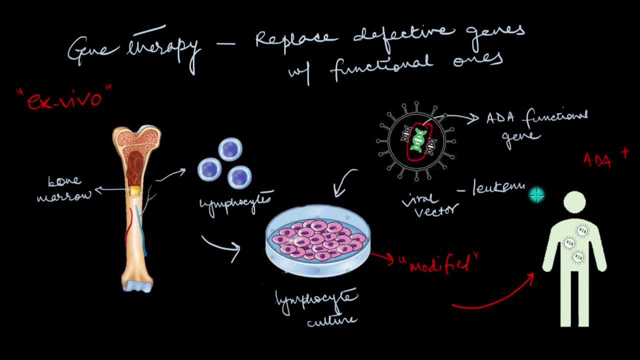 gene could not do. However, no matter how cool this entire process seems and it seems pretty fancy and we're getting rid of the problem and stuff, this entire thing was again not a permanent solution. Because, think about it, Because these lymphocyte cells, they are not immortal. 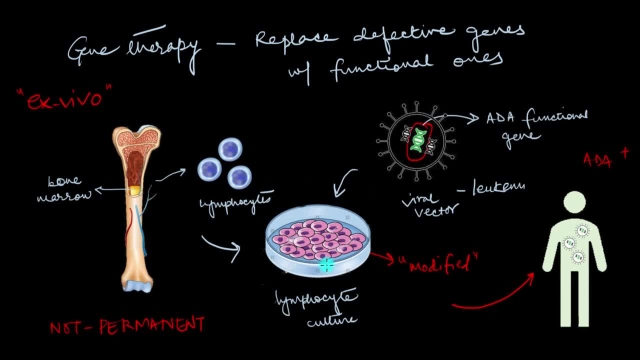 They are not immoral. They are not immoral, They are not immortal. They're going to die, They're going to perish at some point, right, And then what's going to happen Then? these functional genes, these functional ADA copies that we had added, they would also 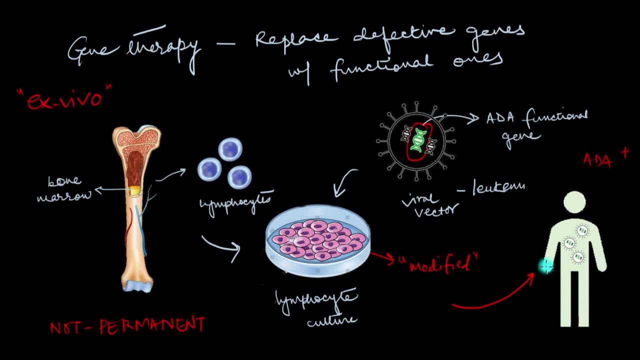 die off along with the cells. So this person will need yet another jab of these modified lymphocytes that we had cultured in the lab, these lymphocytes with the ADA gene, with functional ADA gene, And then he's going to need another because those lymphocytes are gone. 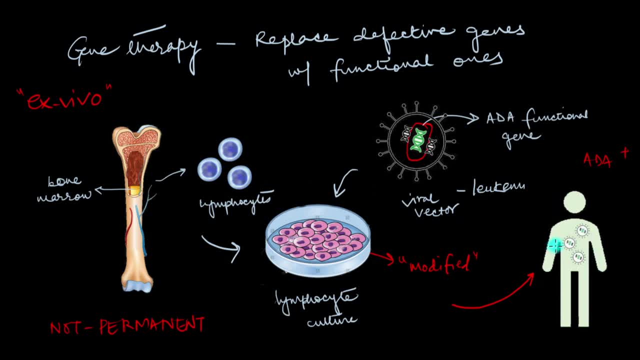 Those lymphocytes are going to die, And another, and another. So you get the idea right. So it's not a permanent thing. again, It's not. Then why exactly are scientists calling gene therapy so promising? If it's not giving us any permanent solution, then what's with all the hype, right? 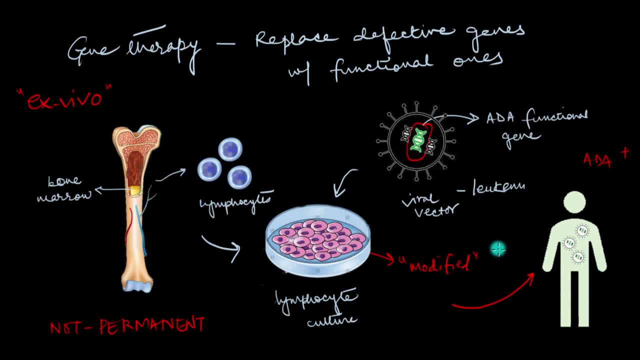 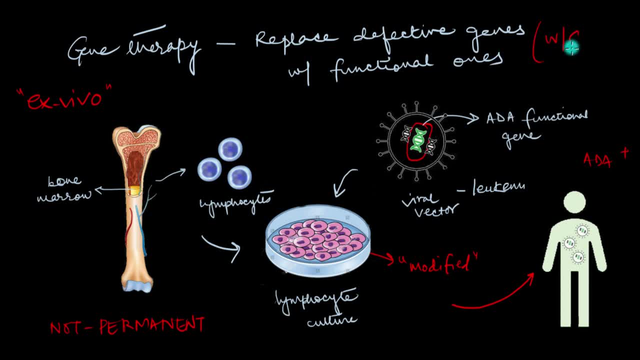 That's because gene therapy has shown evidence. It has shown an excellent result, almost permanent results, with stem cells. Now, we already talked about stem cells earlier, right? So these cells can grow into a very specific type of cell. So when scientists try to do gene therapy with the stem cells, that would eventually 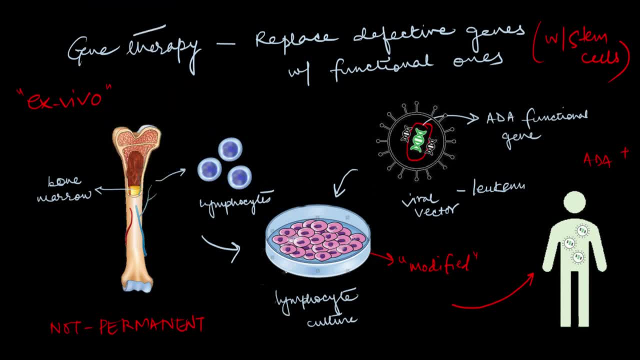 grow into lymphocyte, something that we can find in the bone marrow. like we had seen earlier, You find these stem cells that can grow into lymphocytes eventually, and you can find them in the bone marrow. so when scientists tried to do gene therapy with these stem cells, then they saw that this 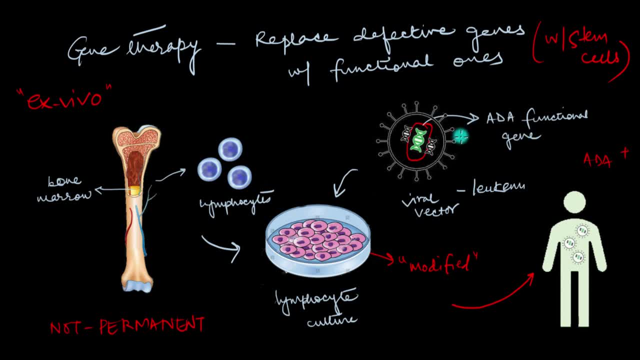 ada functional gene that they had inserted into those stem cells. they expressed so well that the patient's immunity actually ended up improving so much more. like there was apps. there were absolutely no signs of any form of cancer or leukemia or anything else for that matter. their immunity was really really improved and the gene was getting expressed brilliantly. 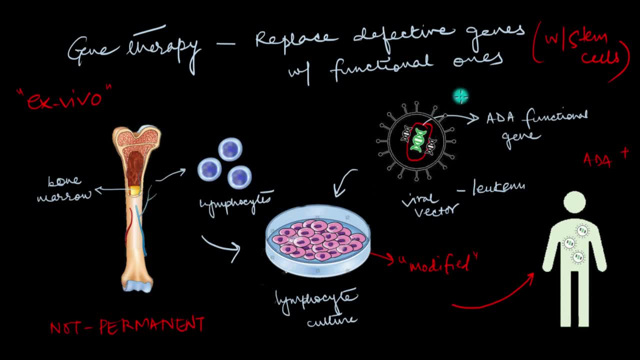 the enzyme was getting produced just fine, almost as good as normal. so that is why we are calling gene therapy promising, because when you are using gene therapy with stem cells they're giving us pretty amazing results, for that matter, almost close, like as close to permanent as we can get. so you see, gene therapy is pretty. 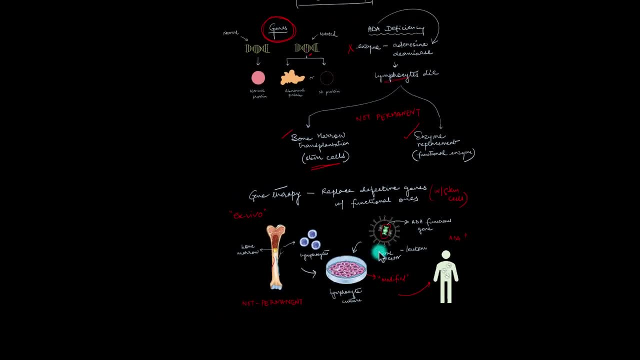 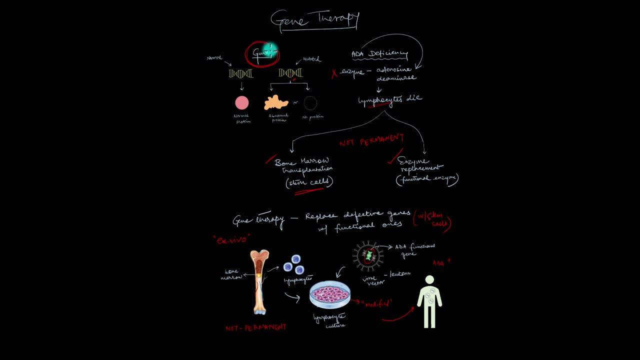 darn amazing actually, if you think about it. i mean, the medical field, science has advanced so much all these years that we are trying to correct genes like genes, not just the symptoms of a disease. that's pretty huge, if you ask me. that's quite huge.